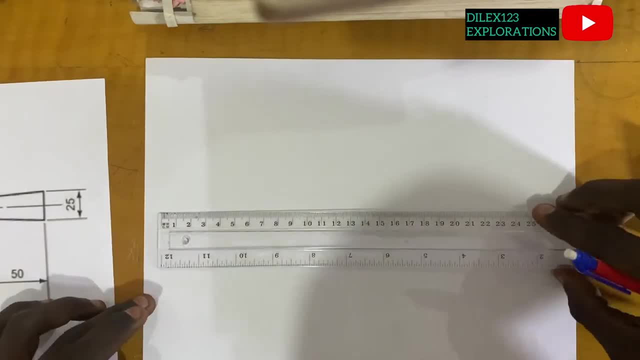 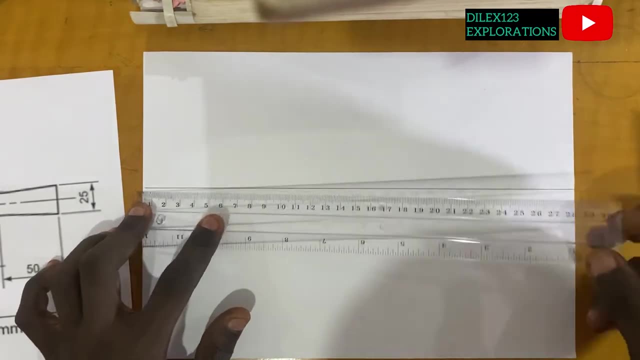 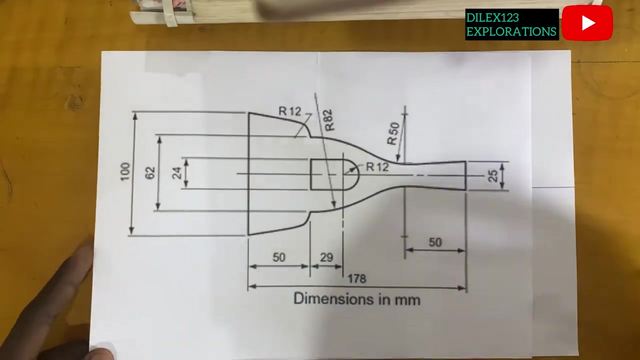 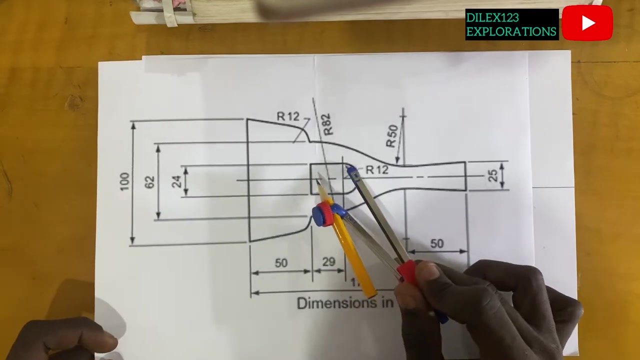 And let's quickly do that, Okay. so, after having done that, the next thing I want to do will be to construct this semicircle Now. R12 means that the radius of this semicircle here is 12.. We can stand at anywhere on the horizontal line. 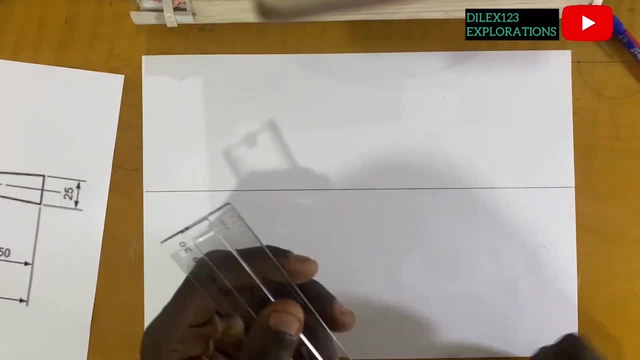 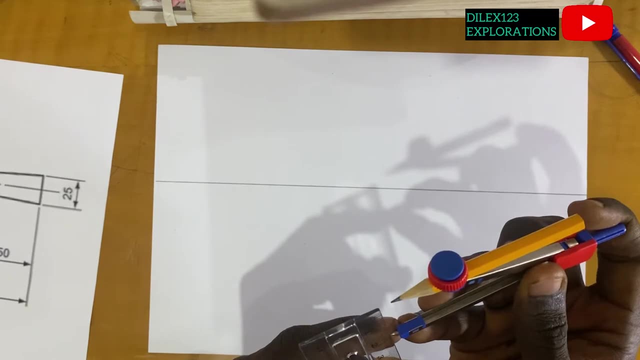 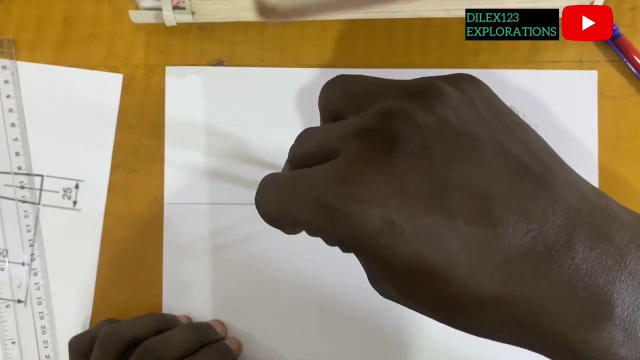 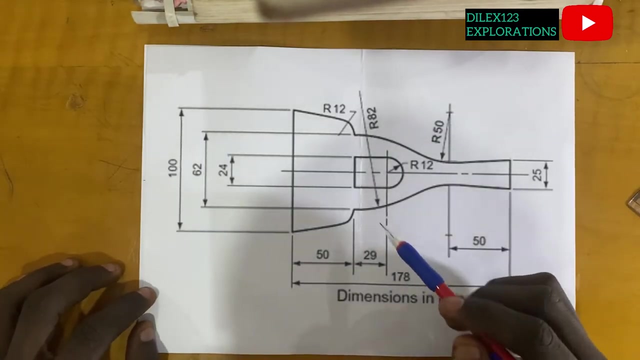 And then we construct a circle, a semicircle with radius of 12 centimeters, So I pick 12 from here. Now let's produce these three lines. So this is a vertical line that is 24 millimeters, And these two are. 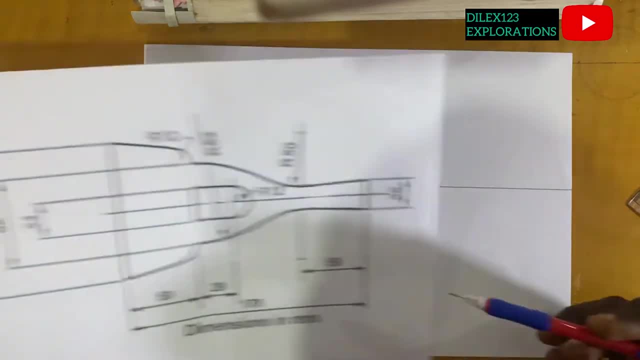 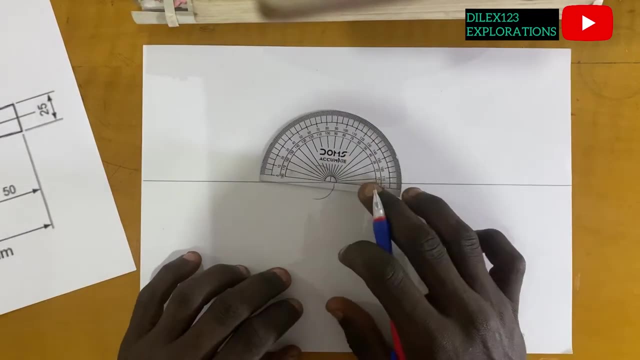 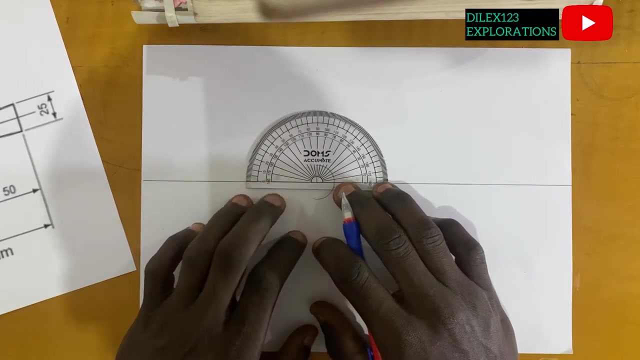 These two are horizontal lines, 29 millimeters each. I'm going to use a totally different approach to do this. I'm going to use this: Okay, so do this, And then I'll pick the 19 mark. That is over here. 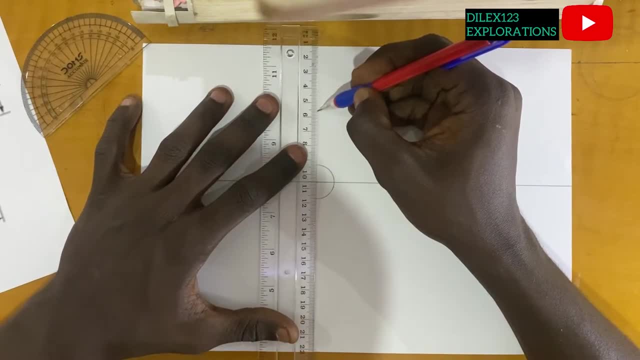 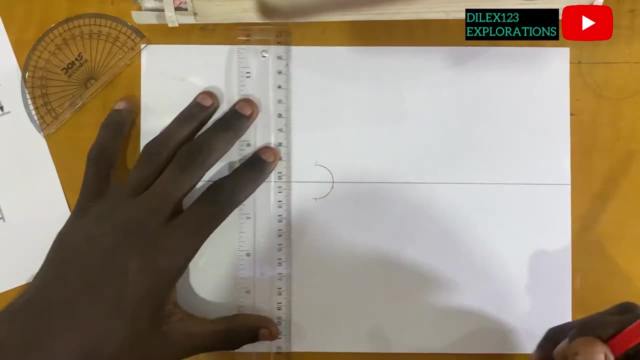 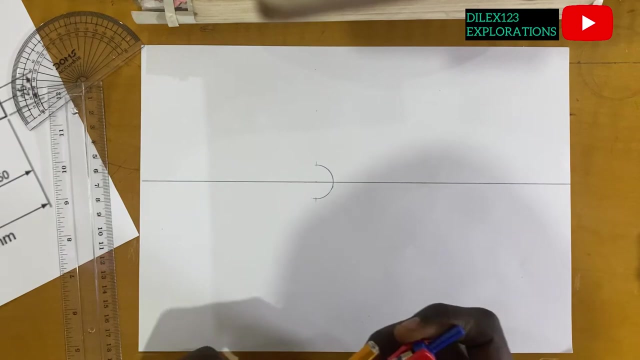 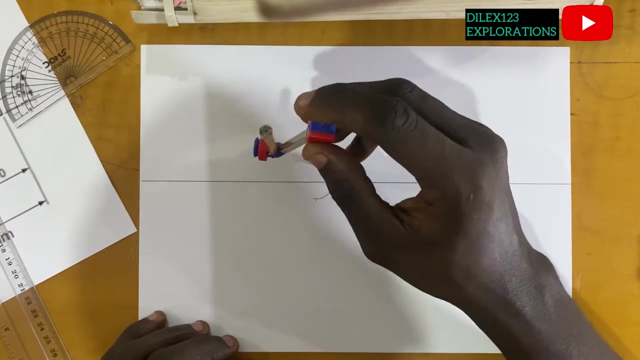 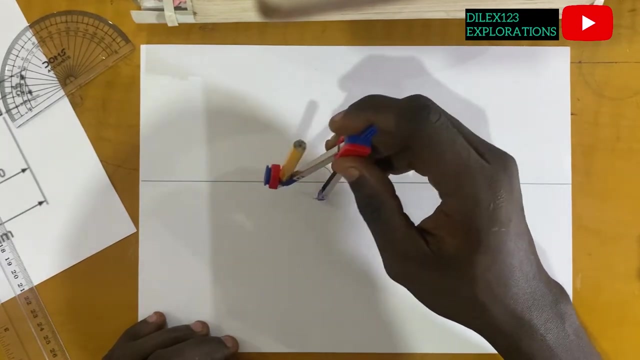 And then I'll mark these small parts here. So I'll stand over here With a length of 29 millimeters, I'll stand here 29 millimeters and mark, I'll stand here another 29 millimeters and mark, And then 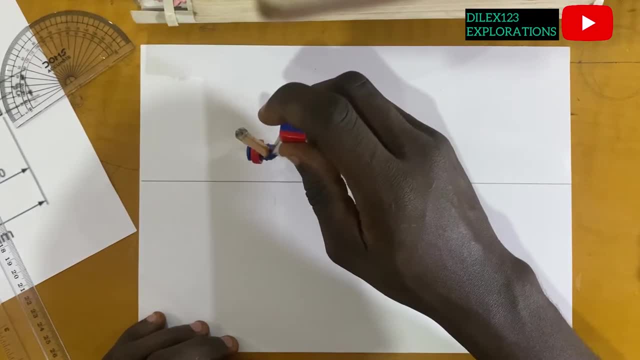 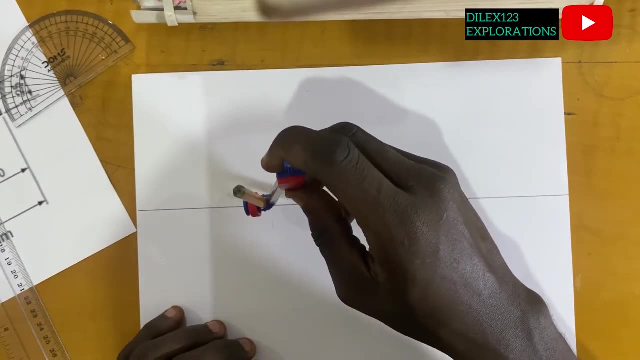 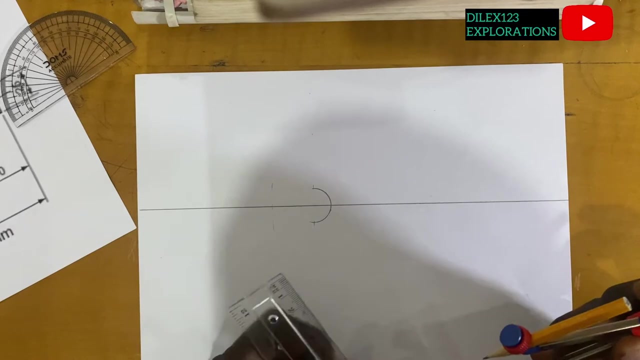 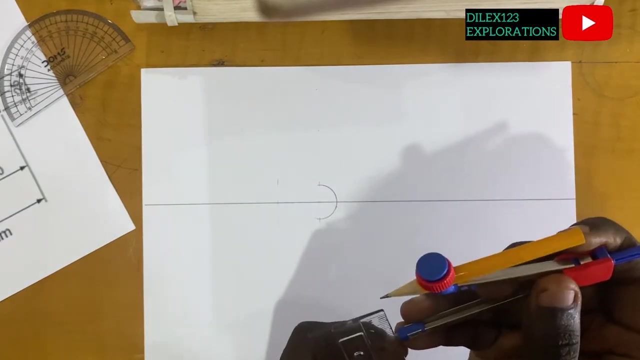 Now I'll repeat the same for this side. The vertical line is 24 millimeters. That means that it's 12 millimeters above and below the first horizontal line we drew. So what we'll do is that we divide 24 into 2 and then we pick 12 millimeters. 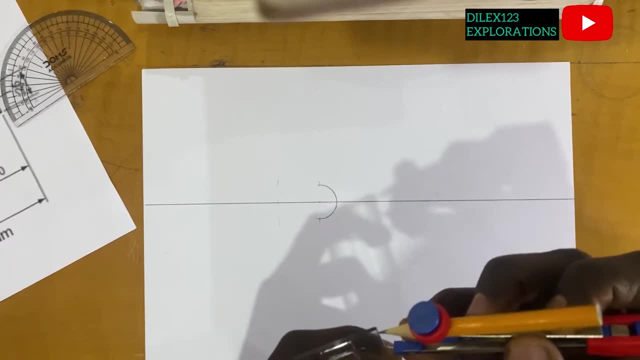 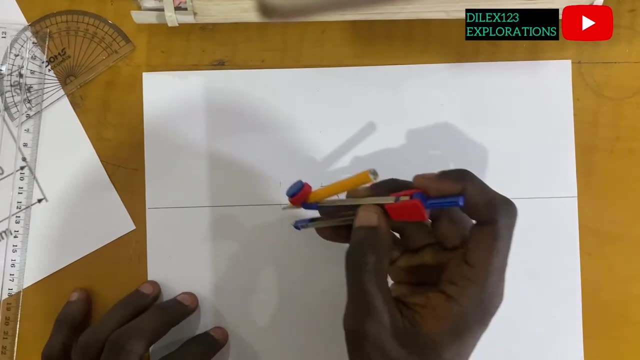 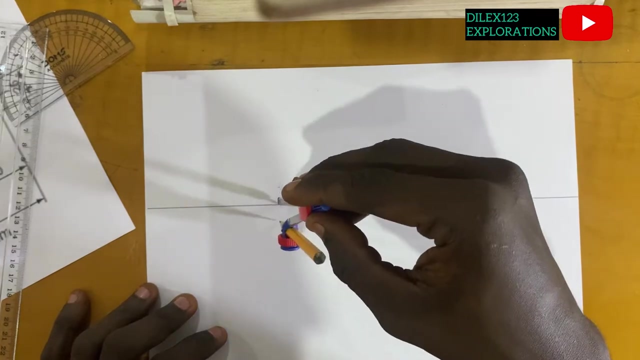 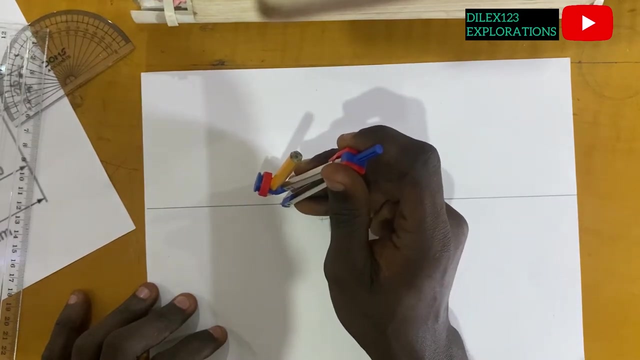 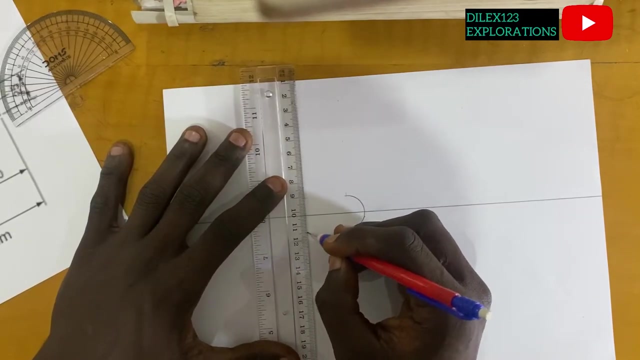 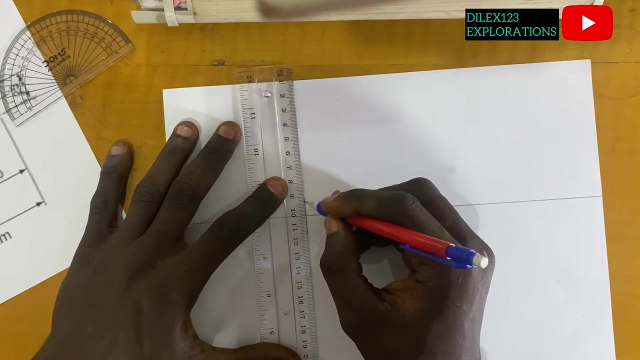 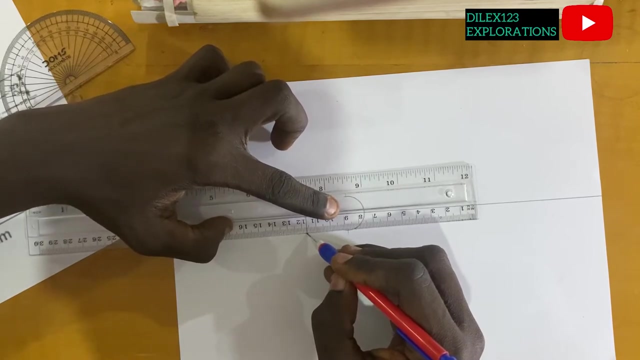 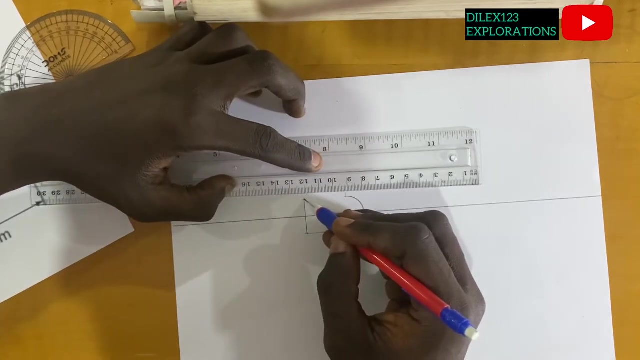 So we take 12 millimeters And then, yes, that is it, 12 millimeters. and then we stand on this first horizontal line with you, and then we mark and we do same below and I link these lines to this and do same for this side. 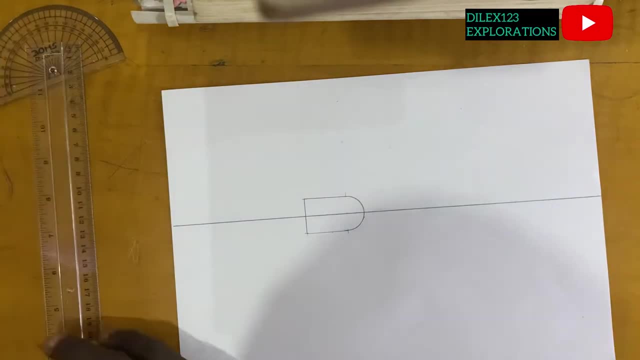 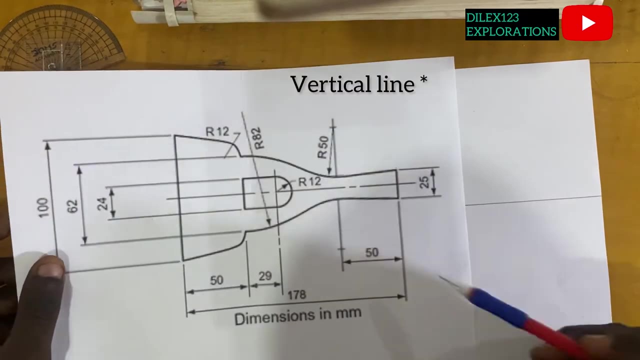 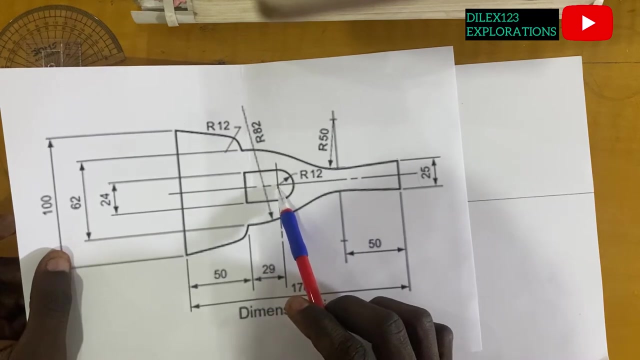 okay, now the next thing that I would like to do will be to construct this 25 millimeters horizontal line, and we can see that this 25 millimeters horizontal line is at a certain distance away from the center of this semicircle. so how do we know the distance it is away from this semicircle? 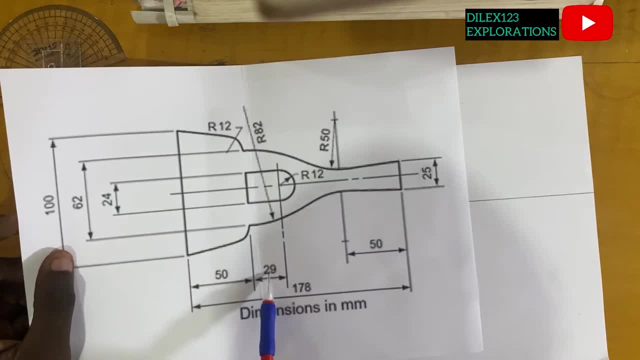 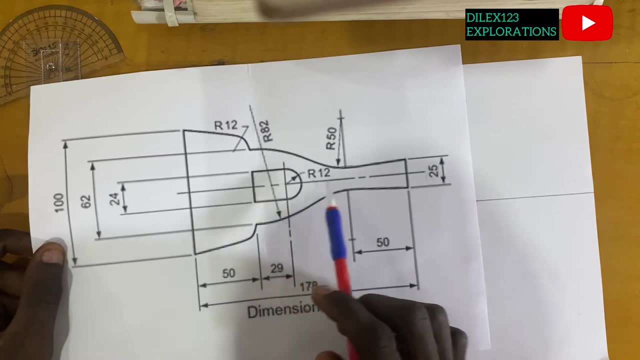 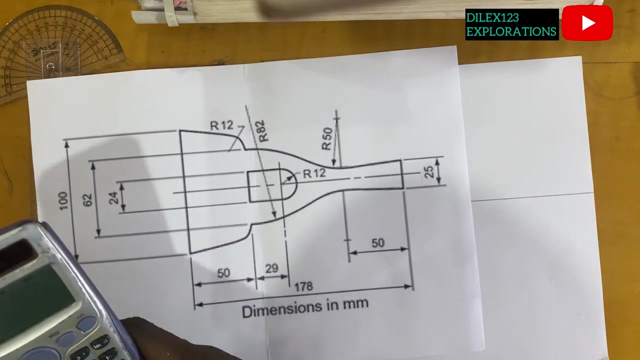 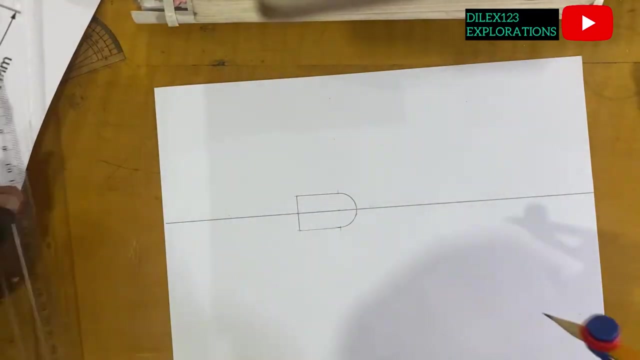 we first have to subtract these two distances, 50 and 29, from 178, and then we'll get the rest of the distance from this side to the end here, and when you subtract to get 99, am i right? 178 minus 79, it's 99. so you pick 99 millimeters from your rule. okay then. 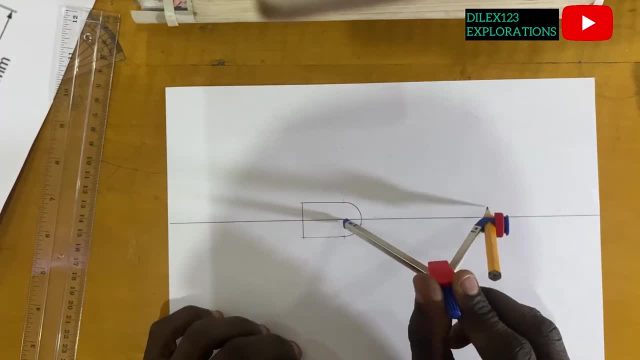 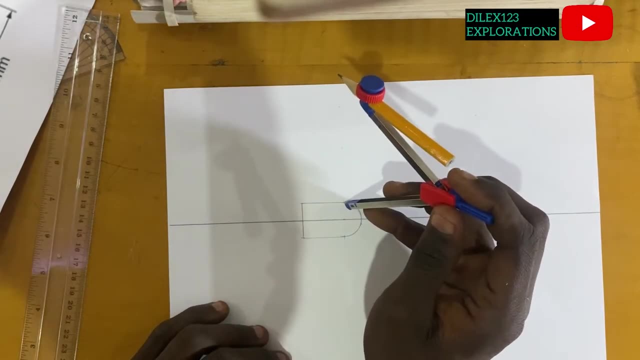 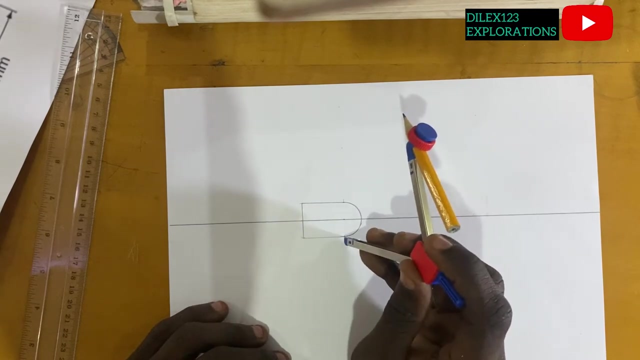 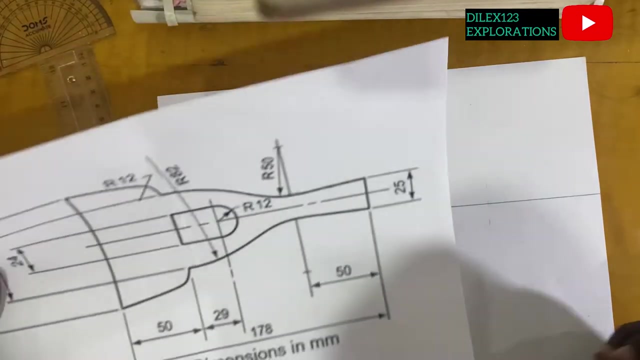 from the center of this semicircle. construct this small arc here. you can do same from the top here, and then also from from the down. here we stand at this point. if this whole line is 25 millimeters, what it means is that from this point, 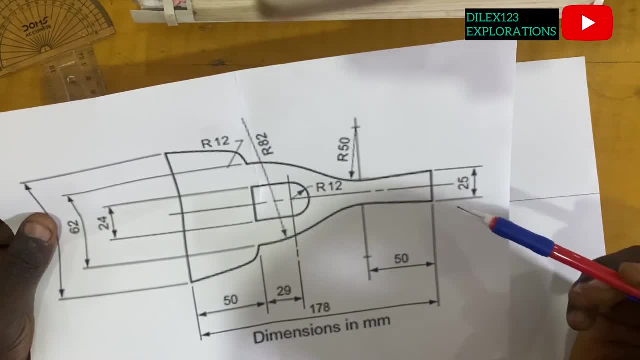 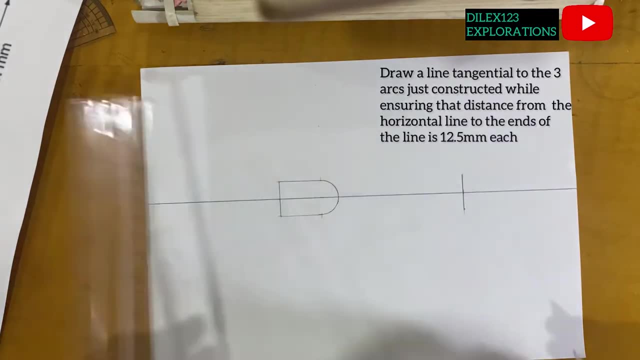 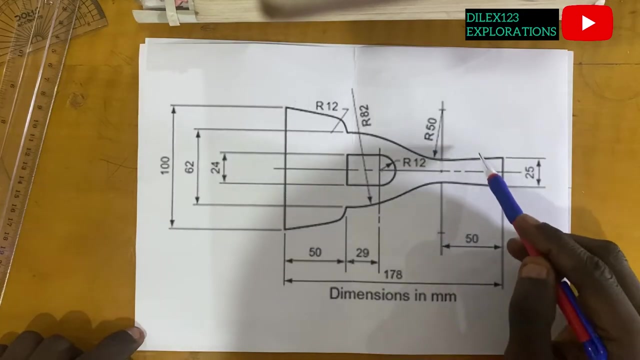 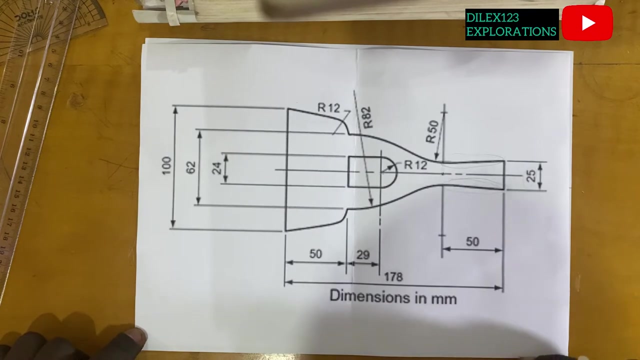 to this edge here. divide: you have to divide 25 into 2, and 25 divided by 2 is 12.5. okay, now the next thing that I want to do is to construct these two lines, but this one is a very tricky one, so let's pay attention and see how we do that now. let's note that from this point over here, 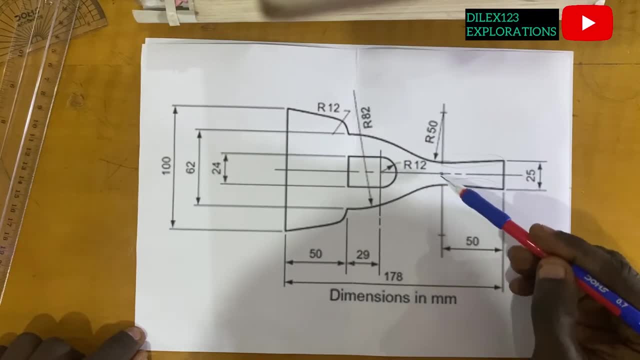 to the point here is 12 millimeters, okay, and from this point below is 12. how do we know that? we can see that from here 24 millimeters and we divide that by 2, we get 12 above and 12 below. let's obtain a point on the center of this semicircle and we can see that this is the center of this semicircle. 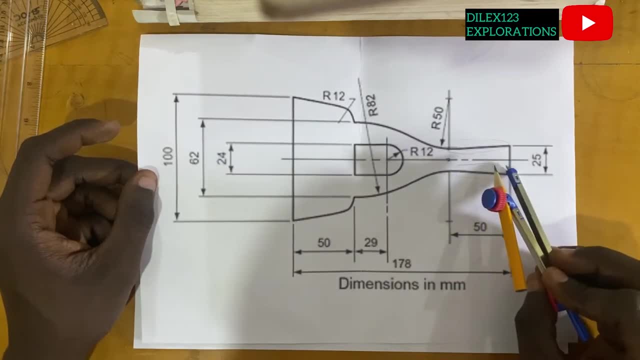 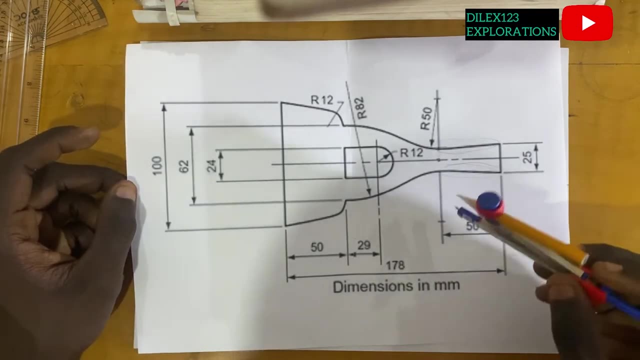 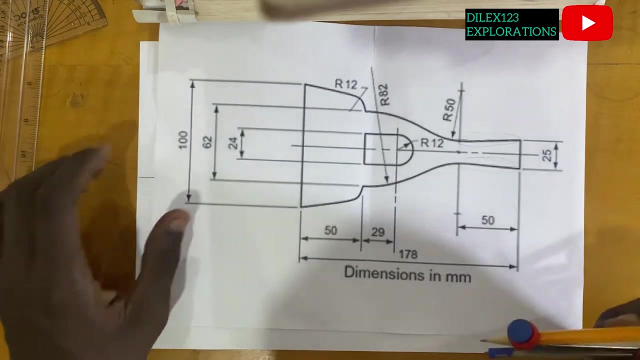 from this horizontal line 50 mm away from this edge here. okay, so after we've done that, we'll construct with a radius of 12 millimeters at that point that we obtained. with the radius of 12 millimeters, we constructs acts above and below the point, so I will first of all have to pick 50 millimeters. 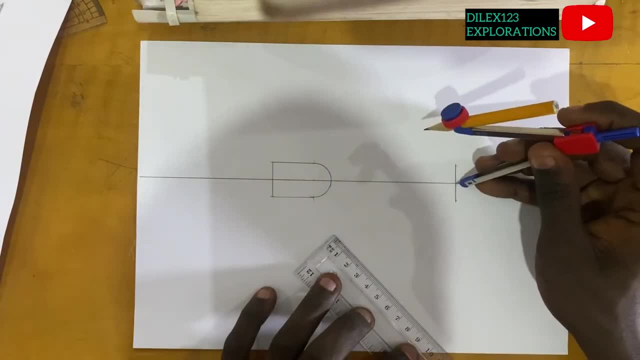 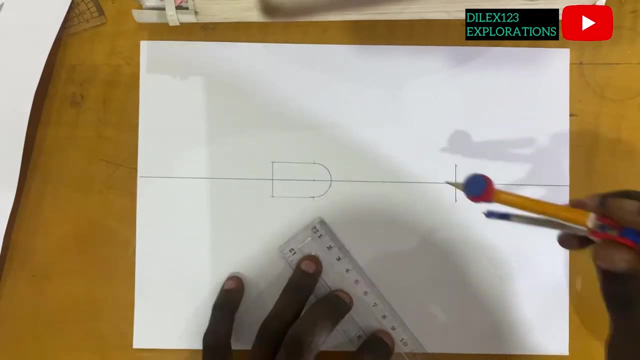 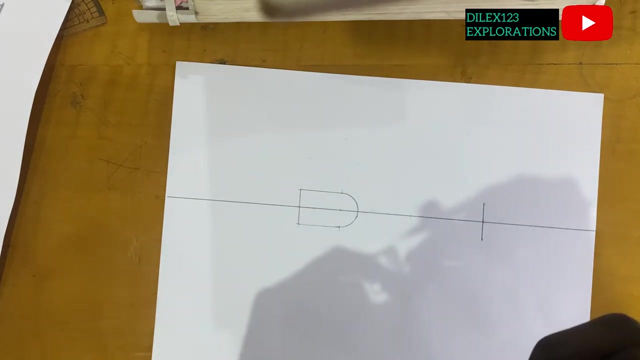 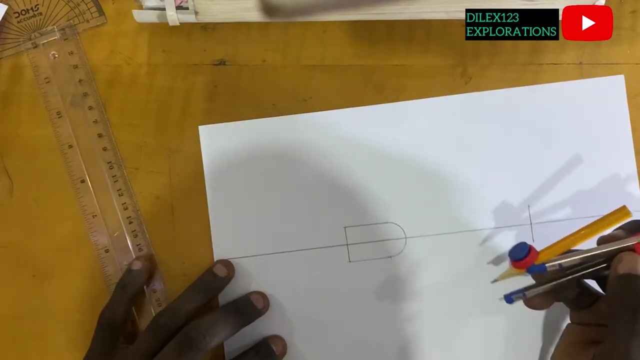 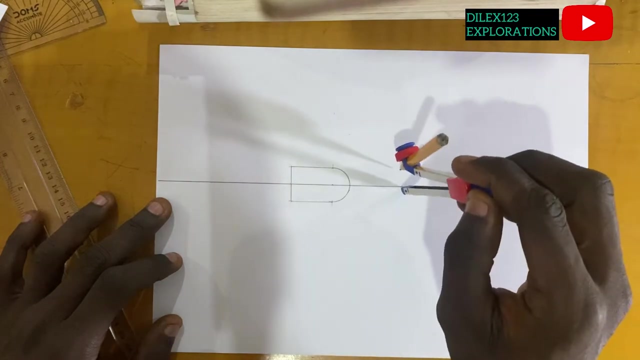 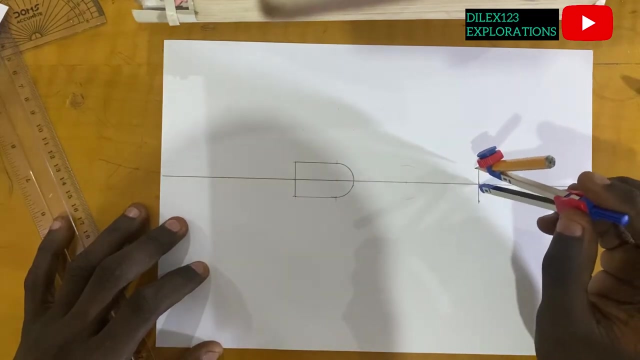 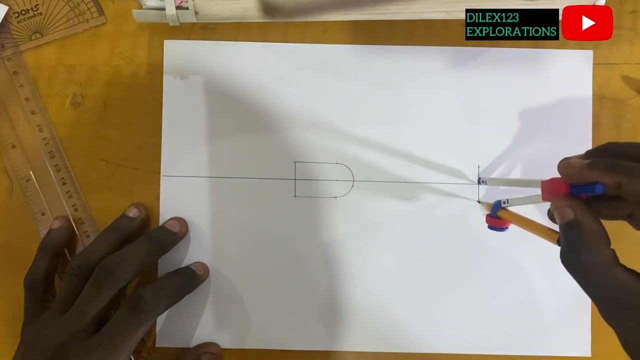 from my rule. okay, so stand here, right here, here, right here Now. what I will do is that I will have to pick a radius of 12mm. then, from this point over here, I construct an axe above and below. Now I also have to construct 12mm over here on this vertical line. 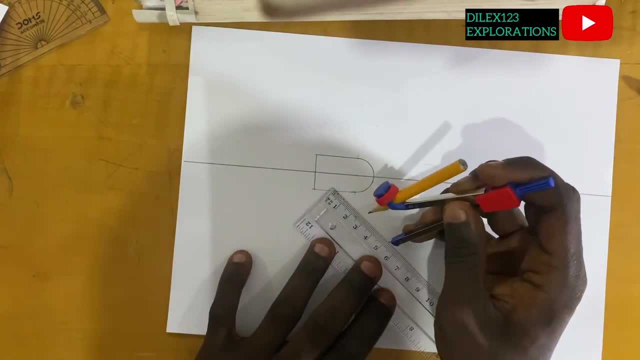 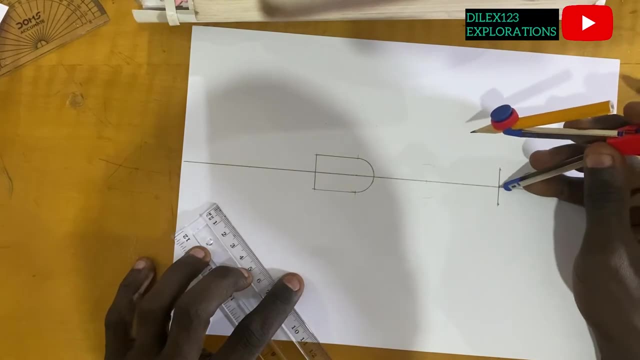 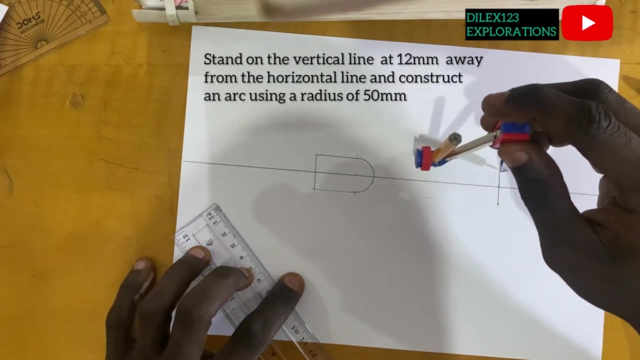 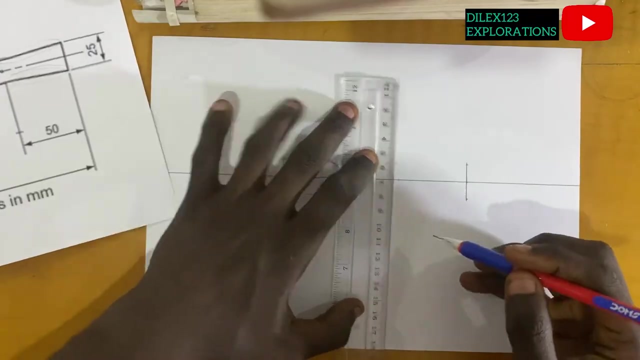 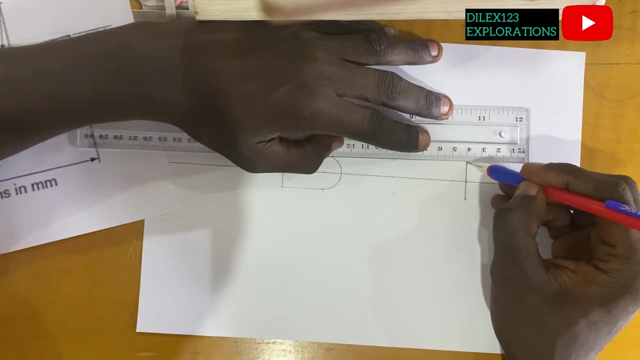 So with the same 50mm that I picked initially. Okay, So with the same 50mm, let me see if it's still the same thing. okay, Then I stand below here and do this. Okay, so I'll join the top here to this side, and the line should be very visible. 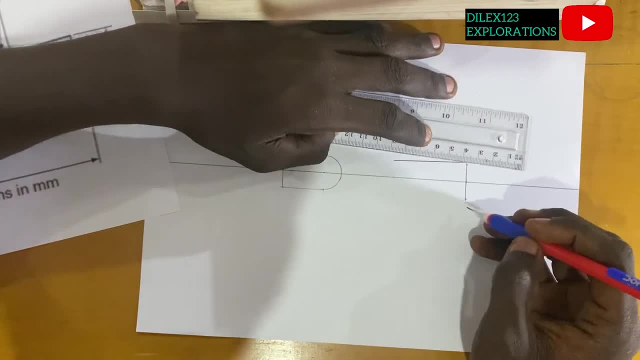 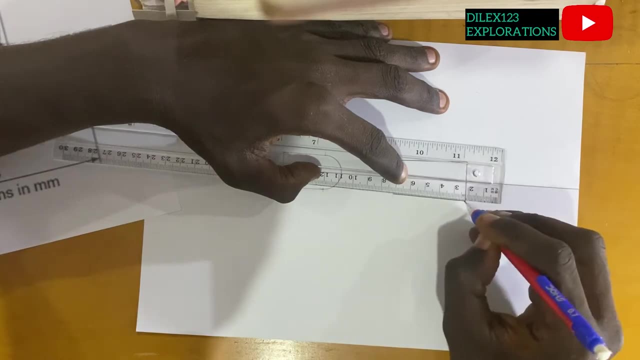 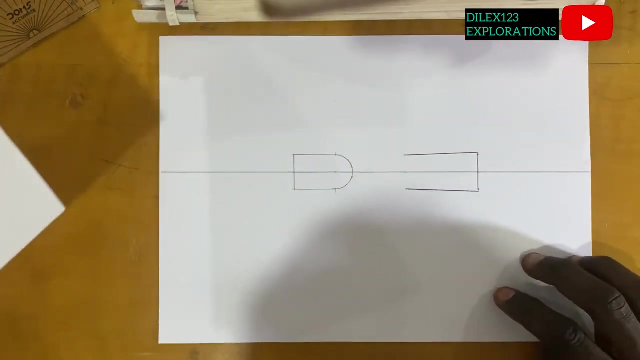 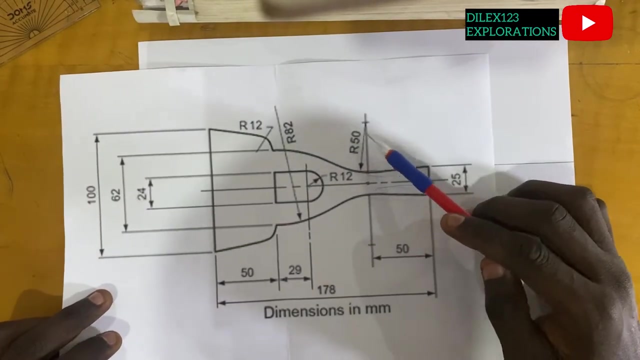 Okay, And then I do the same for this side. Okay, We can see also from the diagram that there is a certain circle over here and that circle has a radius of 50mm. So with the same 50mm we already have. 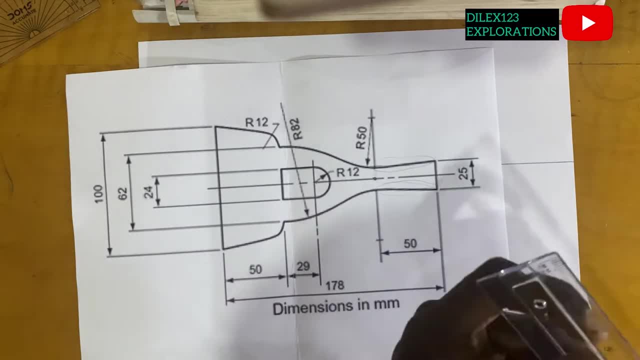 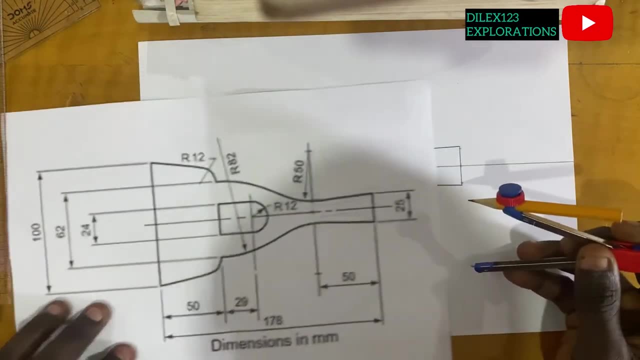 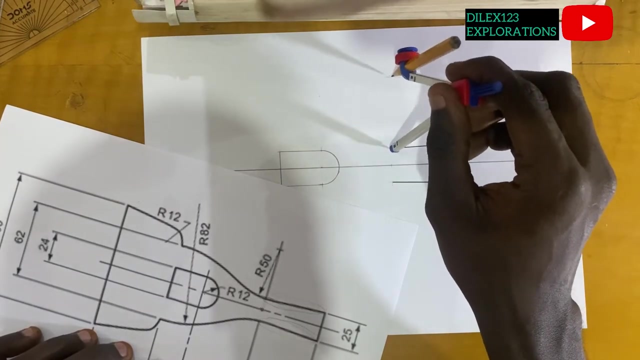 Okay, So I'll join the top here to this side. Okay, We'll have to try to be able to construct that circle. And what do we do now? You stand at this point. we now have you construct 50mm above, that's the arc, and you do the. 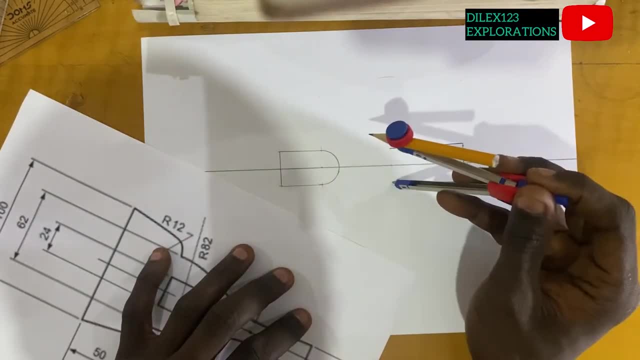 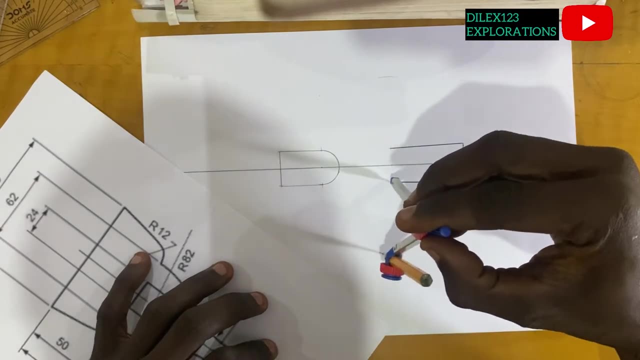 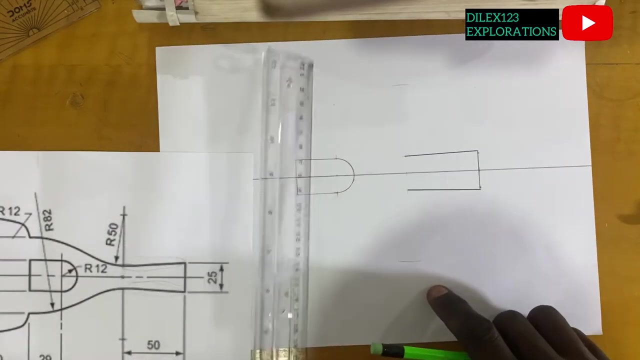 same below. Now you have to stand here to. you have to stand here to do the one below, Okay. Okay Now, in order to get the point of intersection- I'm not really going to stress myself that much- I'll have to continue this line. 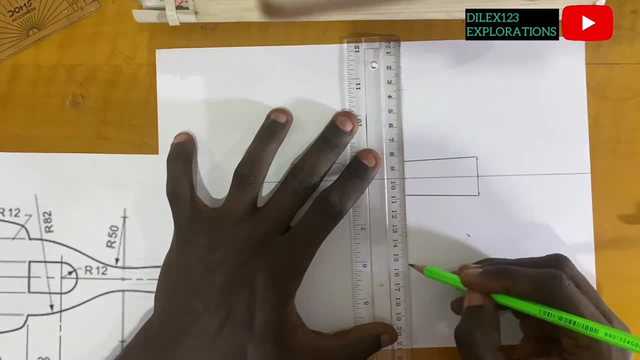 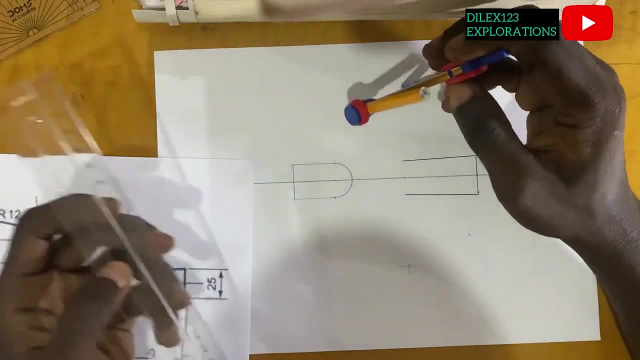 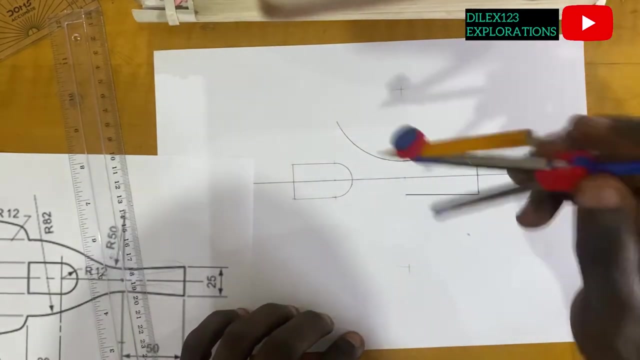 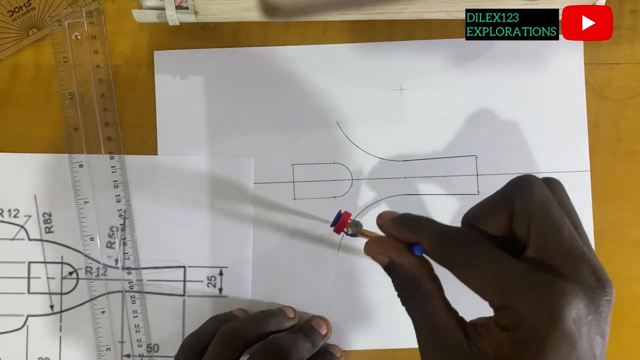 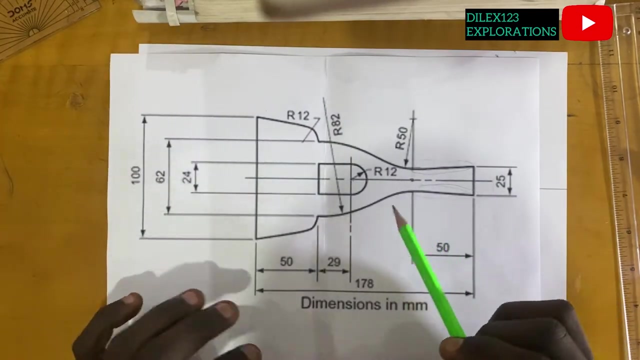 Yeah, so it intersects over here. So what it means is that you stand over here and, with a radius of 50mm, construct an arc. Then we do the same, Okay. Then we do the same below over here, Okay, The next thing now is to draw this arc. 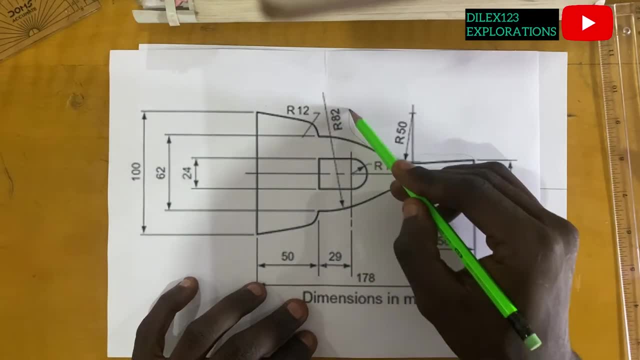 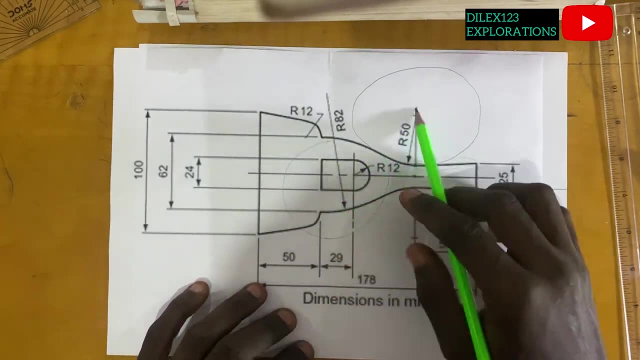 When you look at it carefully, you see that there are actually two circles. This is one of the circles, and then this circle is another one, So the two circles are touching each other, Just that we didn't draw this part of the circle. 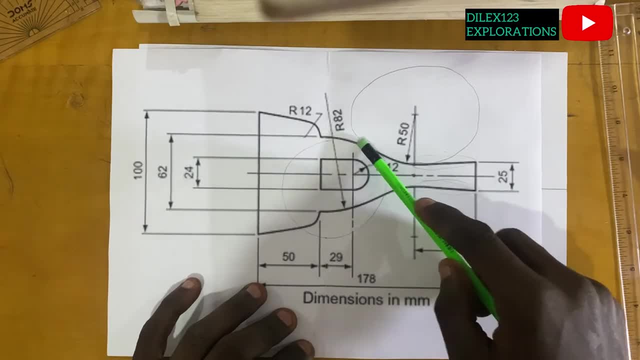 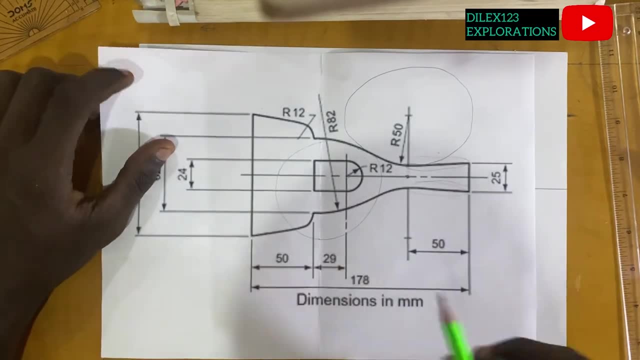 It's in the diagram. We only drew the parts or the points where they were touching each other. It was just a small part of where they touched. Now, in order to obtain a point where you'll be able to construct this arc, you have to. 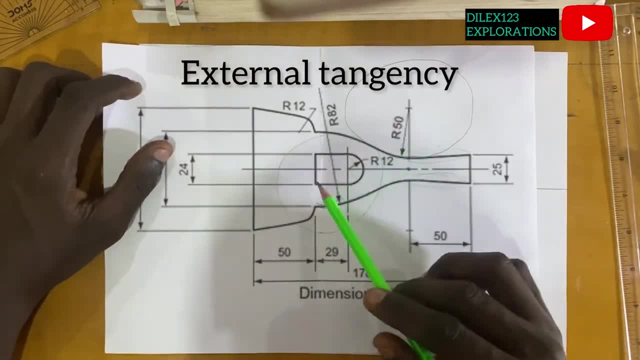 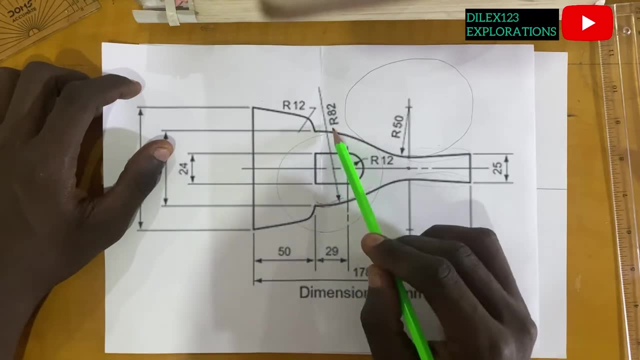 this is called external tangency, because the two circles are touching each other outside. So you have to add the radius of this circle- 50, to the radius of this circle, which is 82. So 82 plus 50 is 82.. 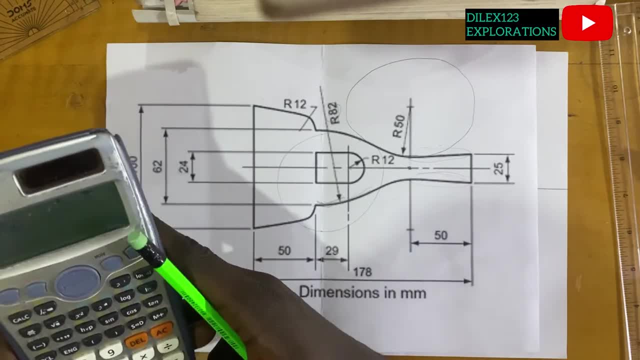 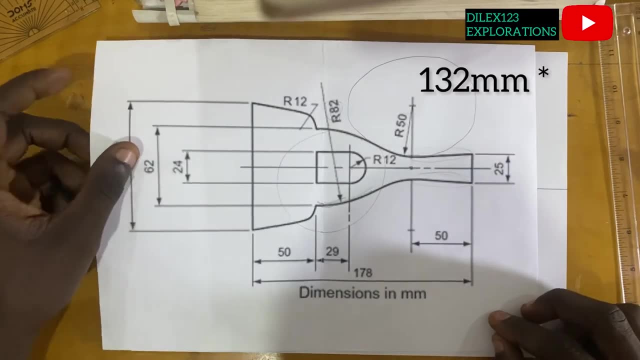 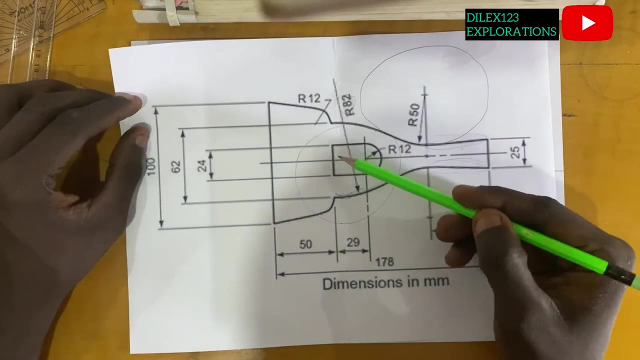 Okay, Okay, 82 plus 50 is 132. So we add the two radii, we obtain 182, and then we would know the points where we should stand to draw the circle. But before we do that, I want to extend this vertical line here, because it is one of the 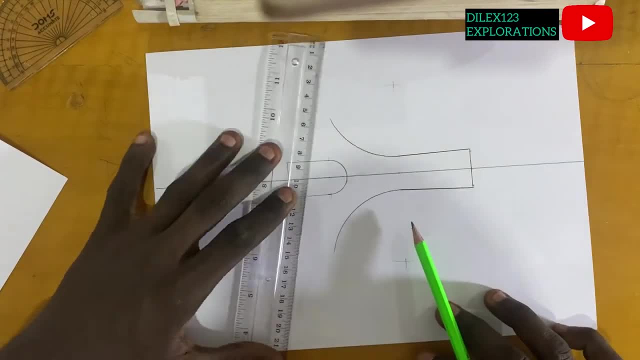 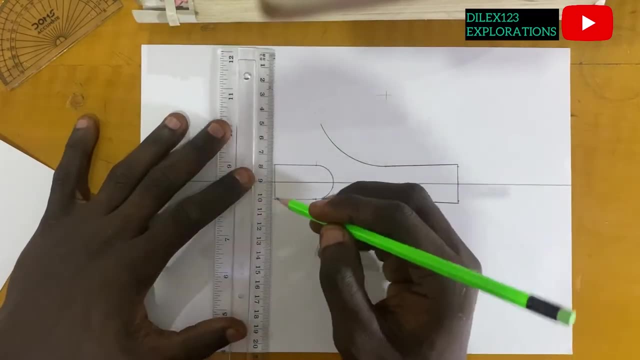 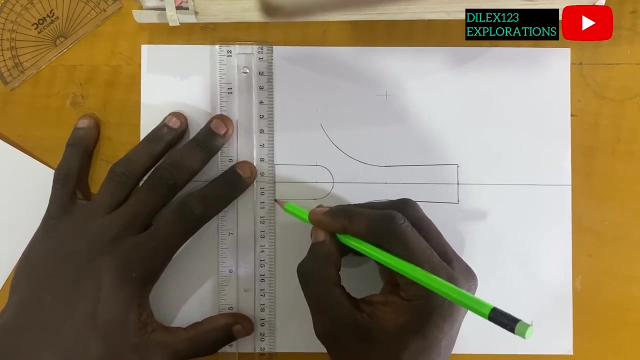 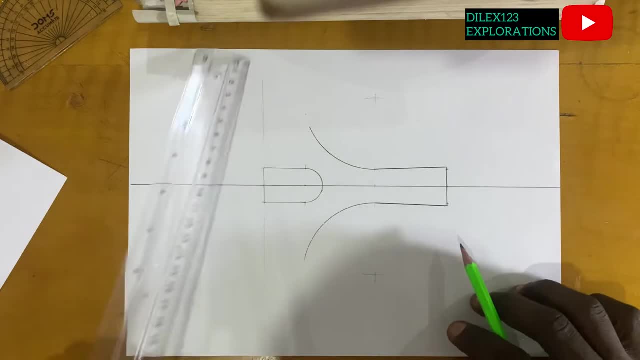 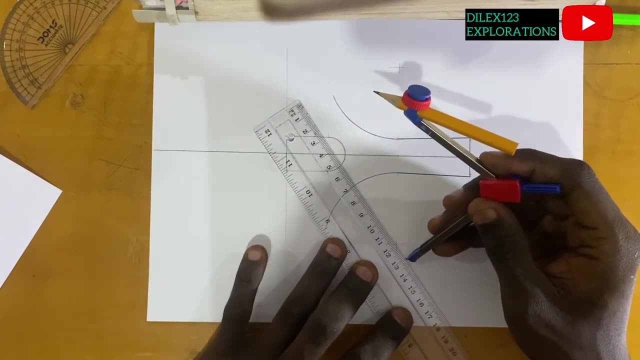 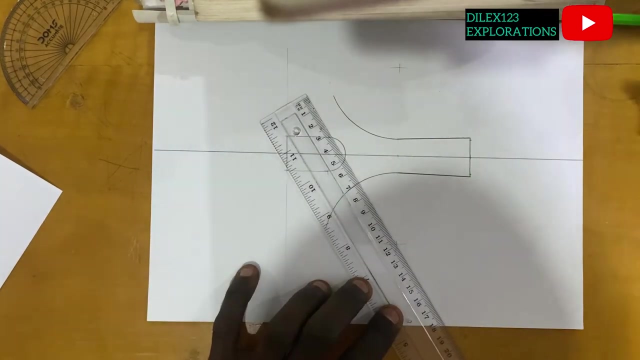 A very faint line Done. Now, unfortunately, I need to pick 132 millimeters, But unfortunately my compass cannot stretch to 132. So, intuitively, what I'm going to do will be: this is the point where I will have to stand. 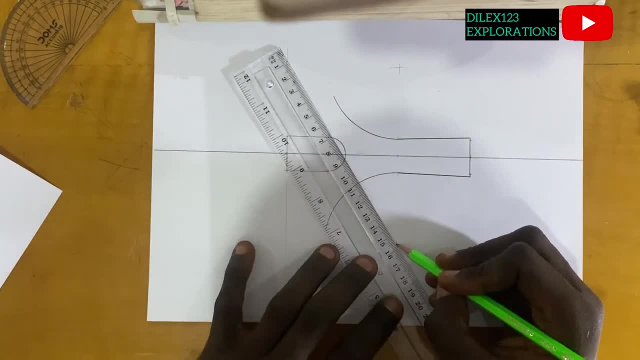 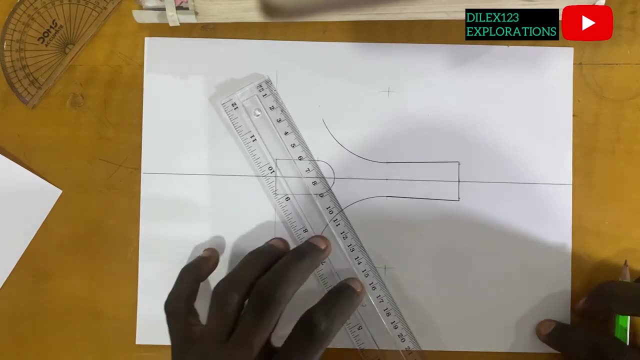 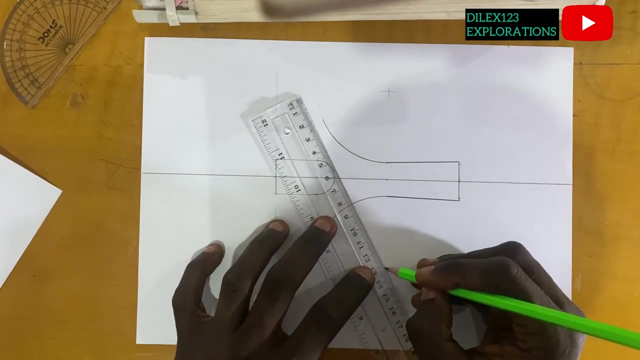 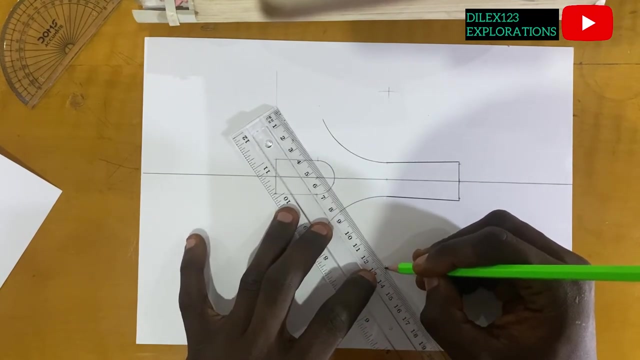 to construct the 132 radar radius. okay, so this is what i'm going to do. interestingly, i'm going to maneuver a way out. i'll stand here and measure 132 on my rule. then i see where i wanted to meet the vertical line i drew. it was exceeded, so i need to come. 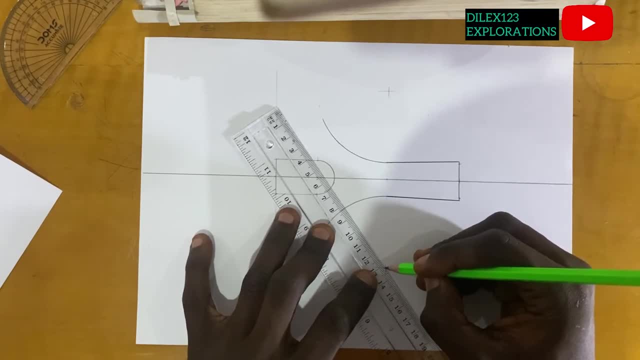 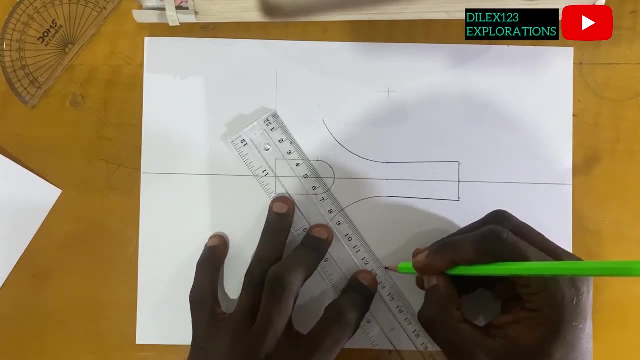 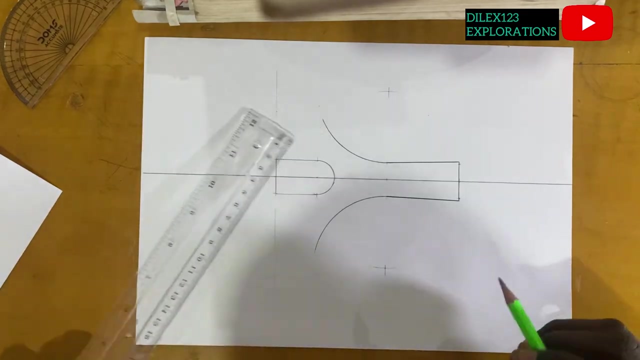 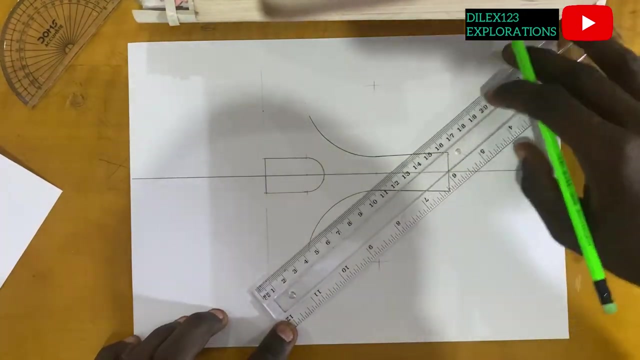 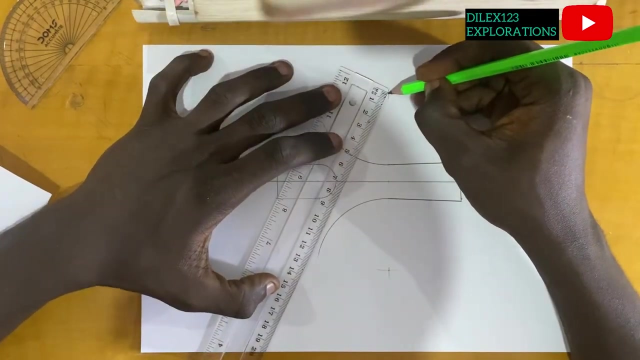 back a bit. so 131 132, i need to come this way. 131 132, this is perfect. so it's meeting over here. okay, now i have to do same for this side, so this is going to be a bit difficult. so this, i need to keep dragging it so it intersects with 132. 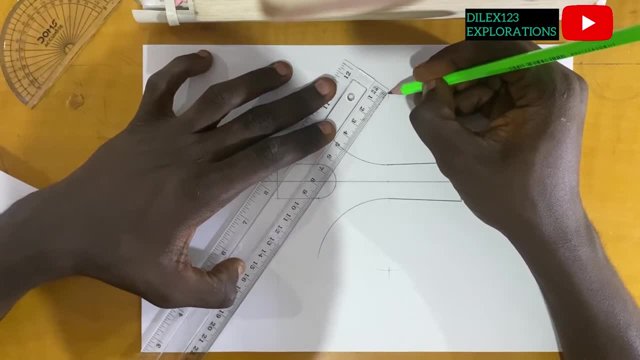 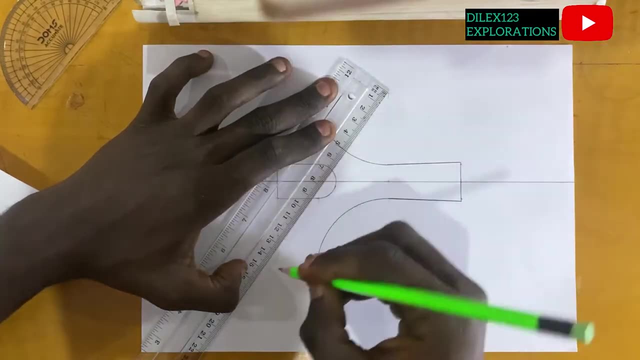 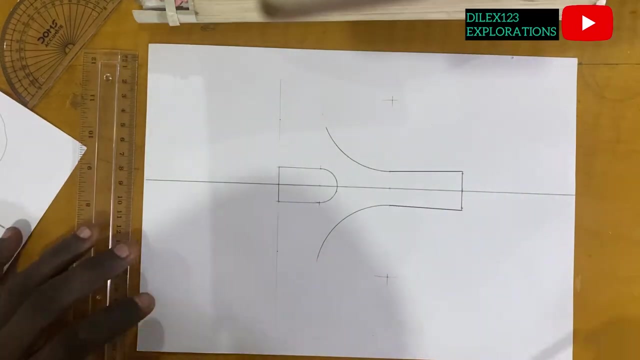 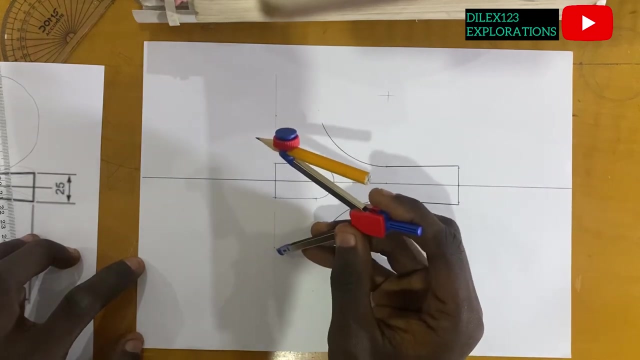 so this 133, 132, then i push this up a little bit- 132 got it here, is it okay? so what i'll have to do now is that i'll just have to stamp over here now with a radius of 82 millimeters, which i've already picked from my rule. 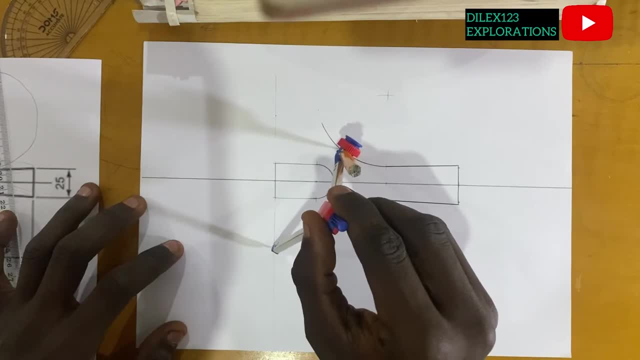 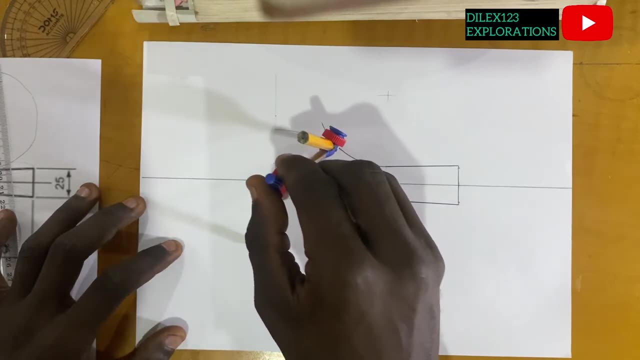 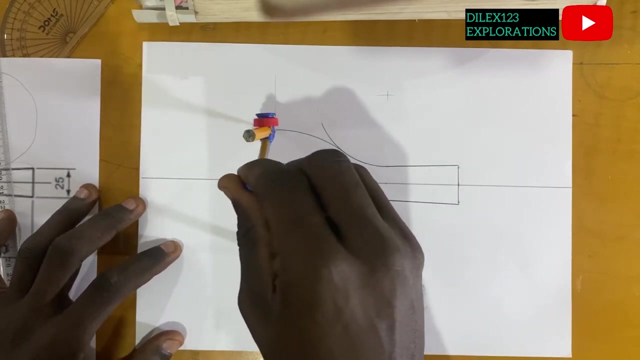 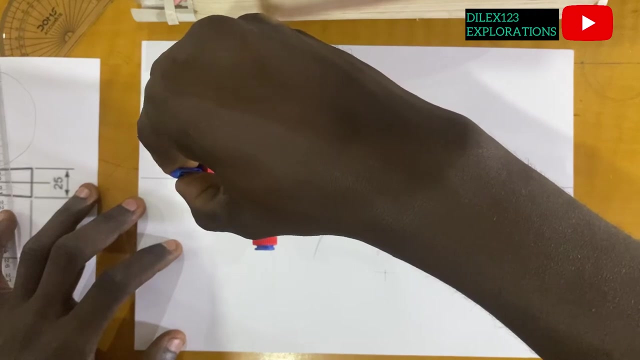 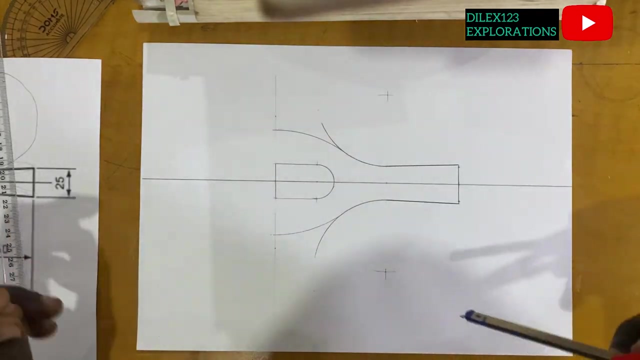 i'll stand at one of these points and construct an arc here, and it will stop at this vertical line. i just want it to be very deep. okay, then i stand at this point also and then do the same, make sure it's still same. you definitely have to clean these lines, but we will do that in the course of the video. 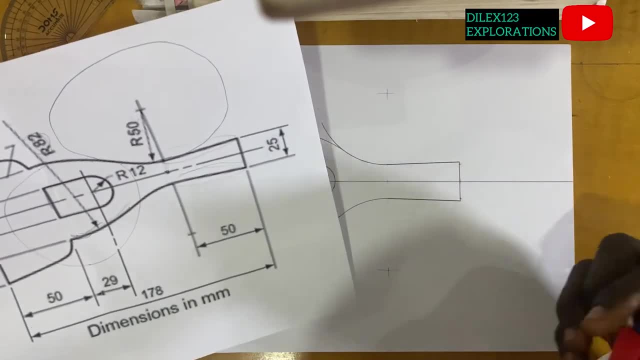 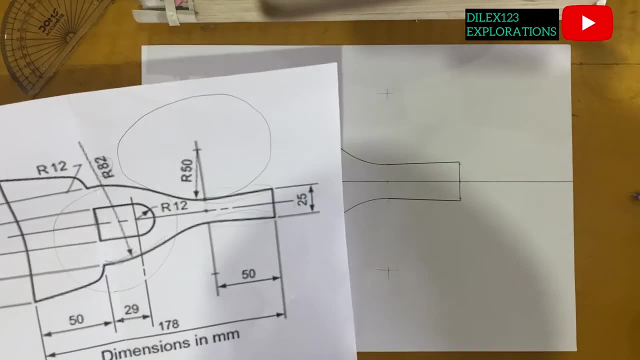 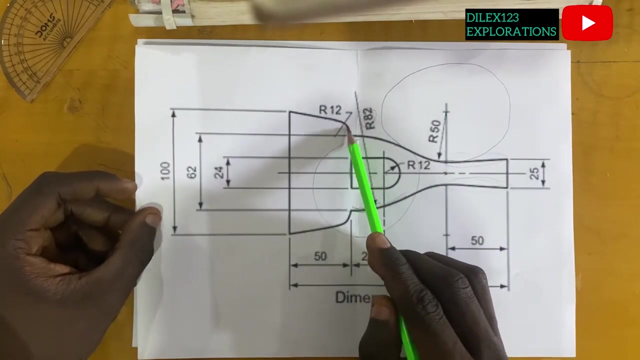 i think that now we can see that our shape is taking from gradually, bit by bit. what is now left is for us to be able to construct this side, and that is pretty simple. what i'm about to do is to construct this small arc. the radius is 12 millimeters, as you can see. 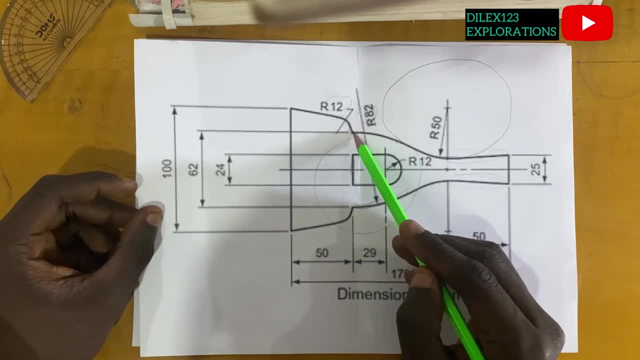 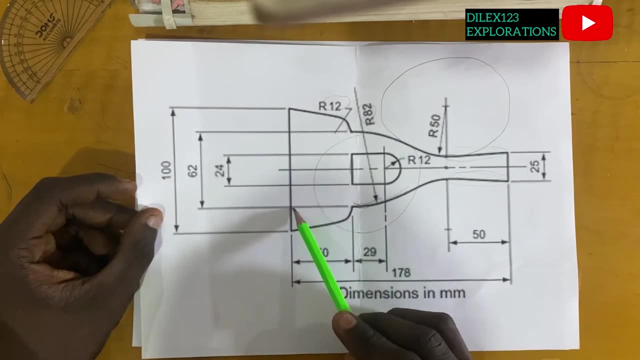 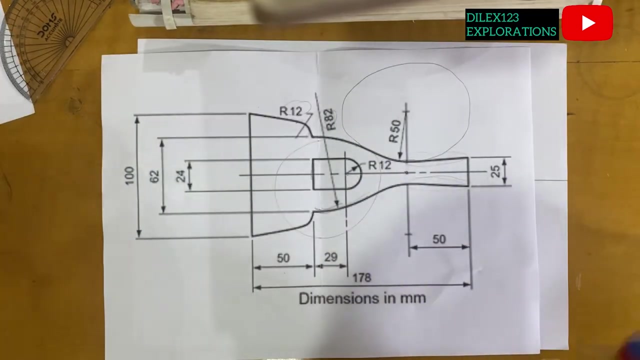 and this i'm going to do it. we can see that from this point over here to the end, here to the edge, here is 50 millimeters. say, it still applies that this points to the end here is still 50 millimeters and this point to the end is 50.. so that's what i'm going to do. i'll pick 50 millimeters from my rule. 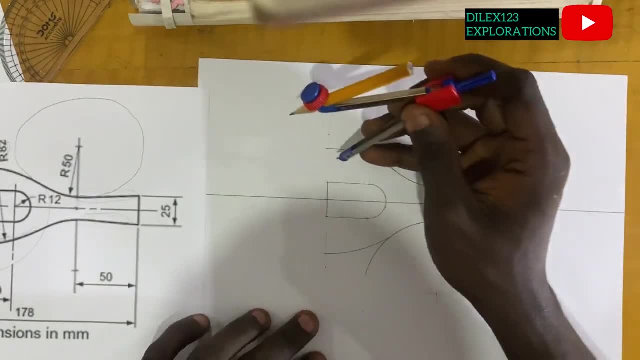 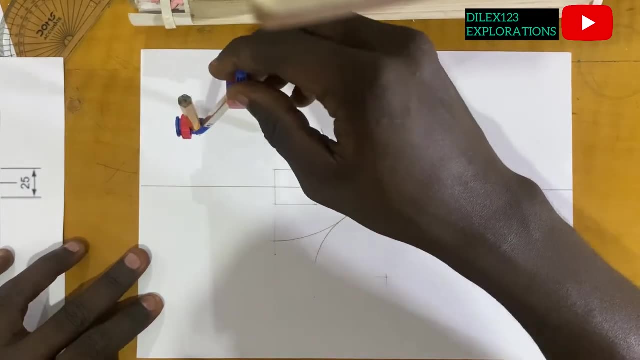 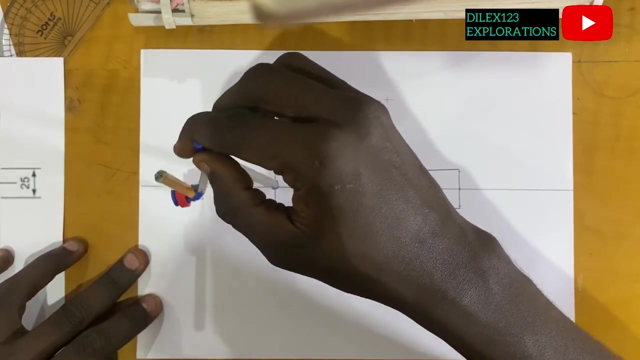 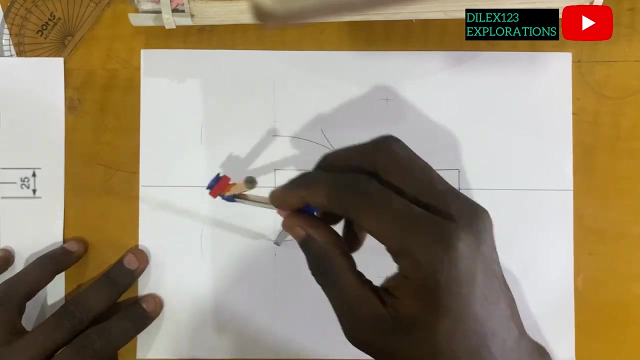 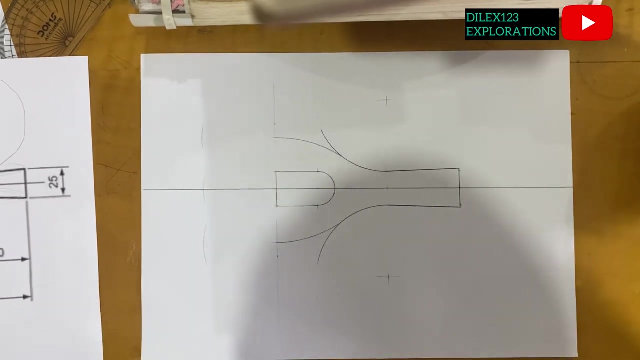 okay, so i have 50 millimeters for my rule. i will stand over here. i'll stand over here and construct this arc. we'll come to this horizontal line, construct another arc and come here, construct another arc. okay, so what i'll do basically now will be to draw a line through that. 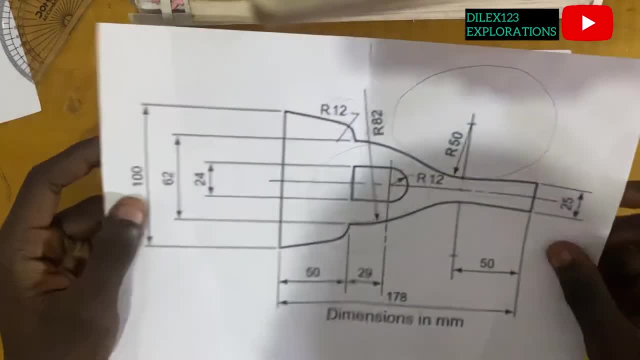 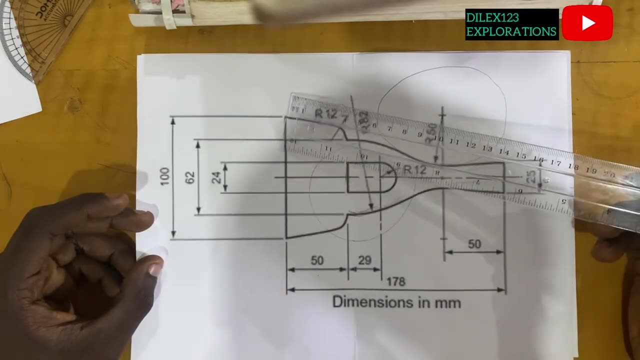 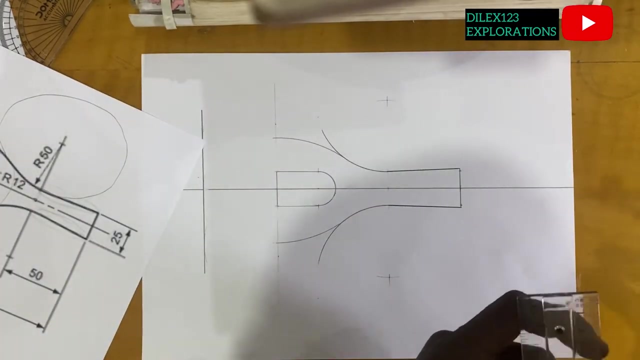 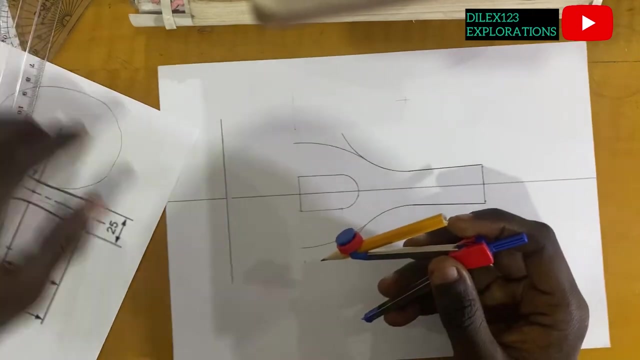 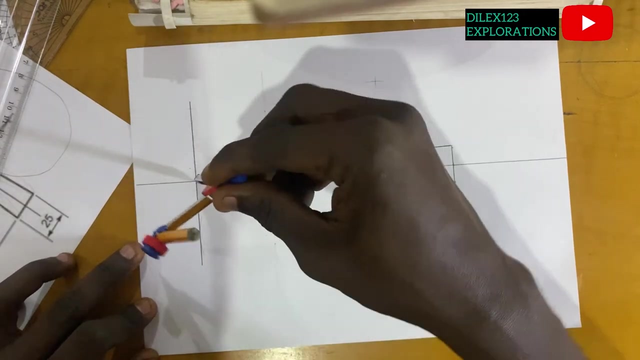 okay, from the diagram we can see that this vertical line is 100 millimeters long. so we divide that into two to obtain 50 millimeters. then we stand at the point where that vertical line meets the initial horizontal line and then we construct an arc. we stand here above. we stand here below. 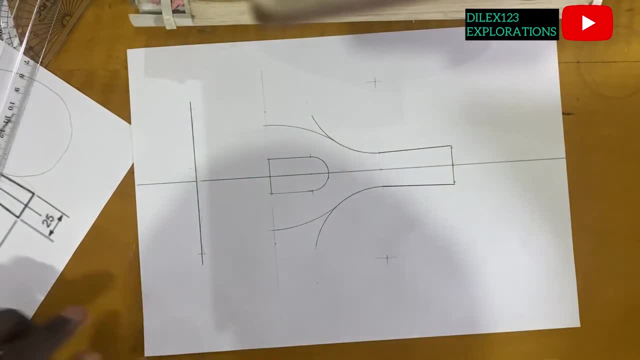 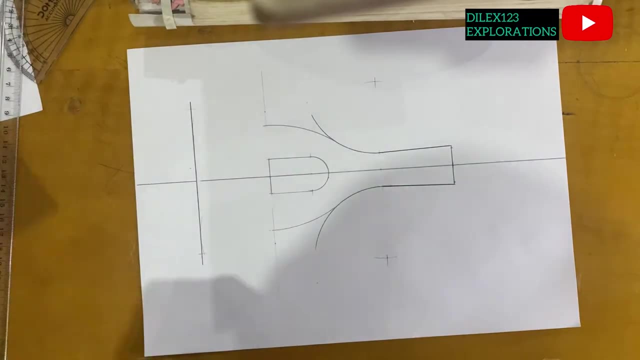 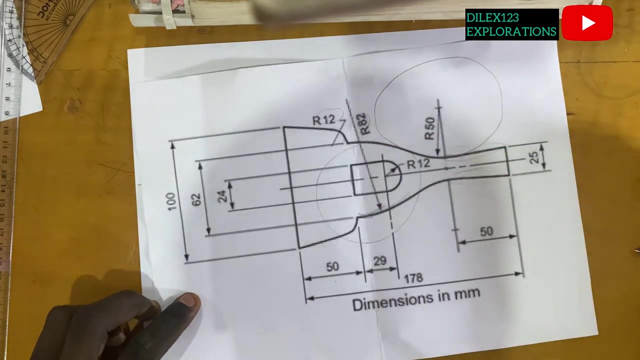 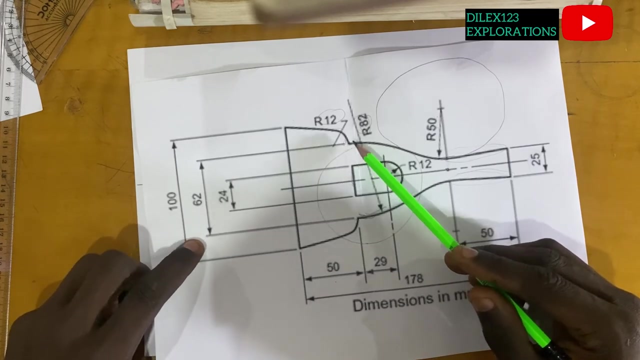 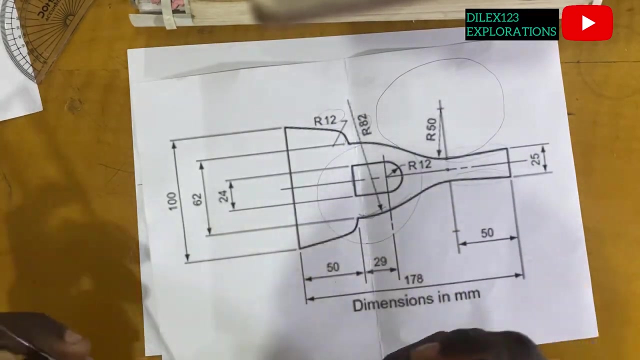 and we will leave that there. okay, now the next thing we have to do is that we can see from the diagram again that this point, this point here, this point here is 62 millimeters long. right from this point to this point is 62 millimeters. we divide that into two, we get 31. so we pick 31 millimeters from the. 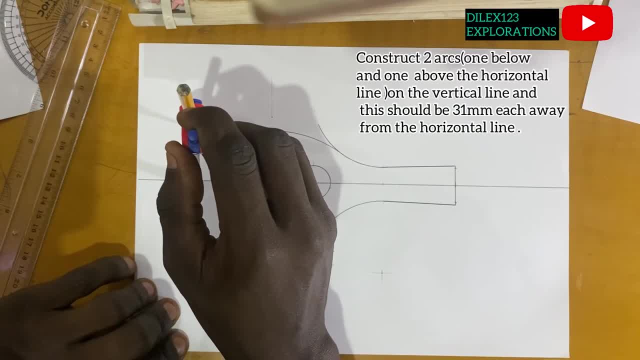 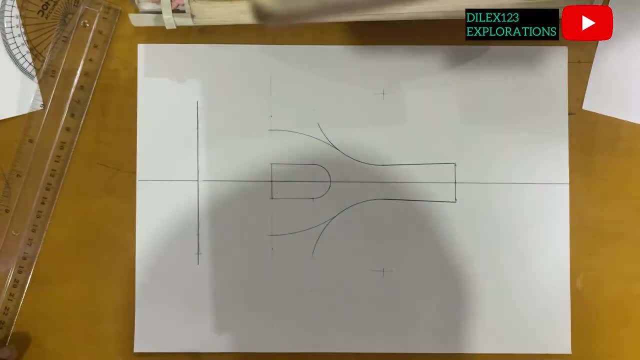 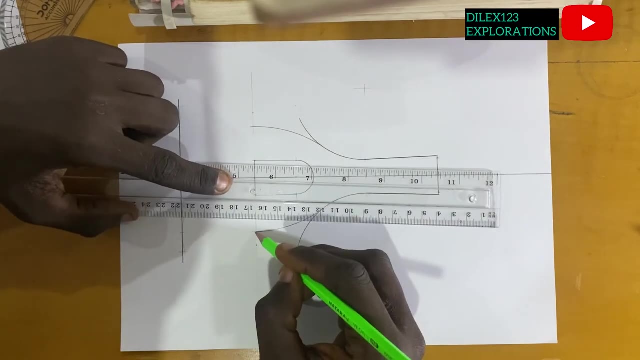 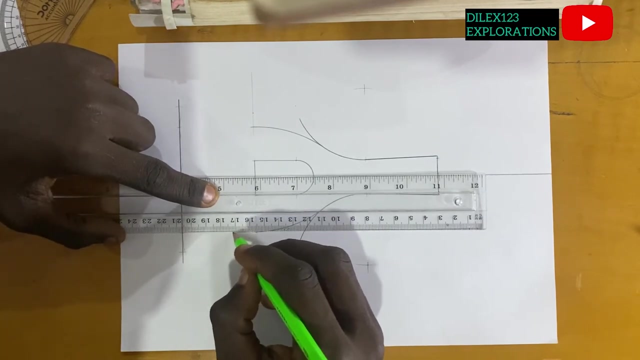 rule, and then we do same below here. now, the next thing we'll have to do will be to join the points, not really as in. you know, join the points, though, but you just want to get at points where we can construct the radius, so you can draw a very faint line. 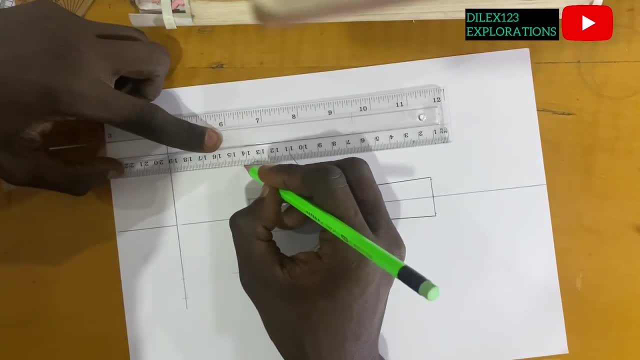 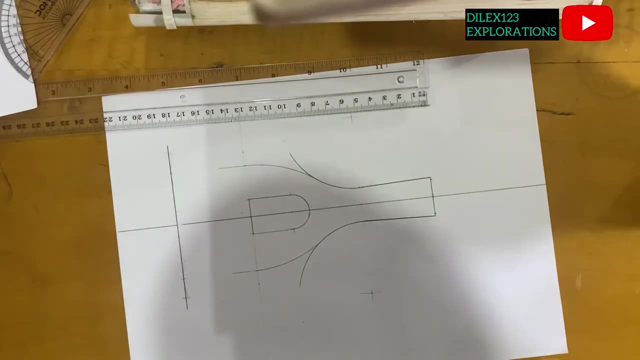 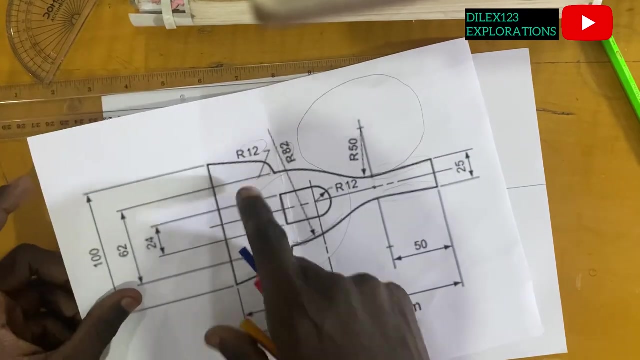 here, and then you do the same over here too. placing too. yes, now we can see from the diagram that the処. now we can see from the diagram that the処, the diagram, that this circle has a radius of 12 millimeters. so we pick 12. 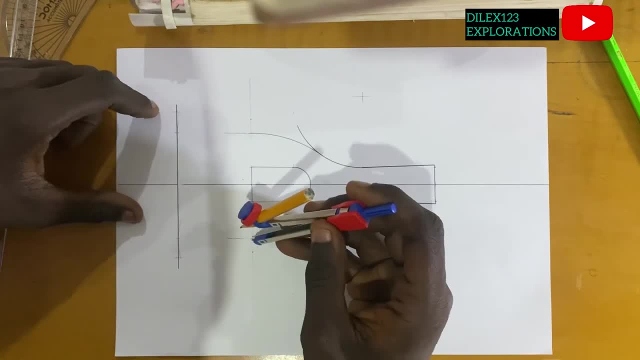 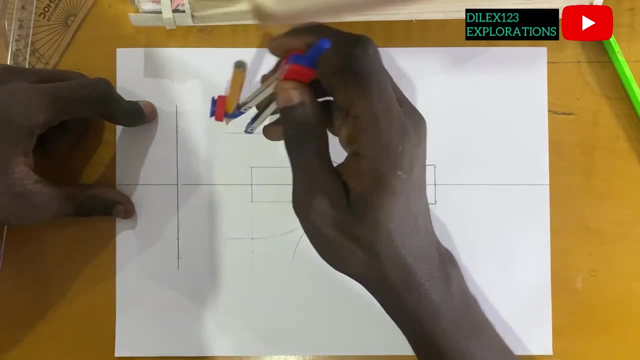 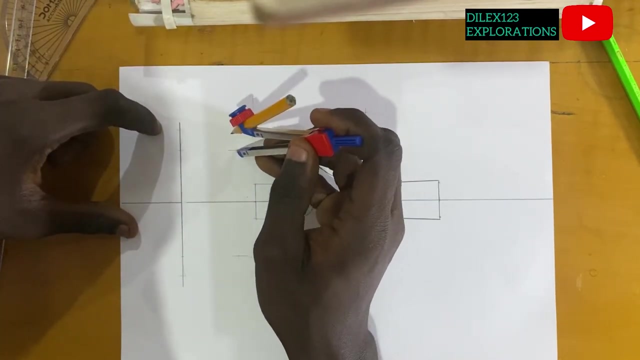 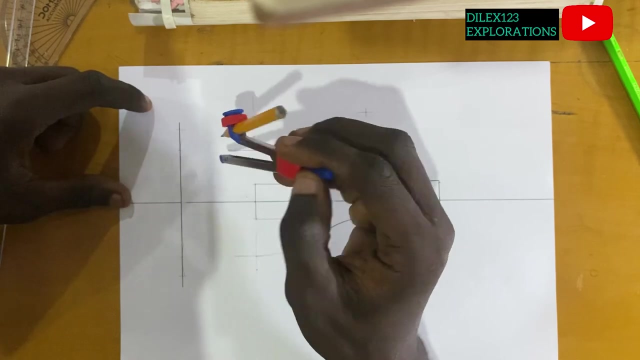 millimeters from our rule, with 12 millimeters, we stand at this point. we construct an arc. we stand at this point. we stand at this point. we construct another arc. now, at this point, with a radius of 12 millimeters, we construct this arc. here we have to do the rule. 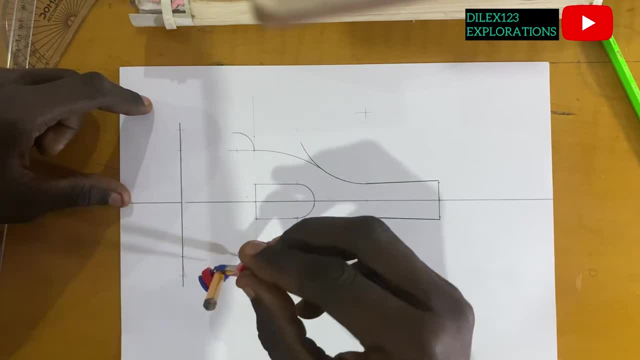 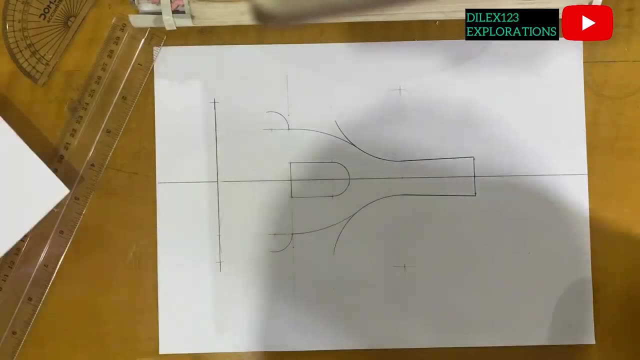 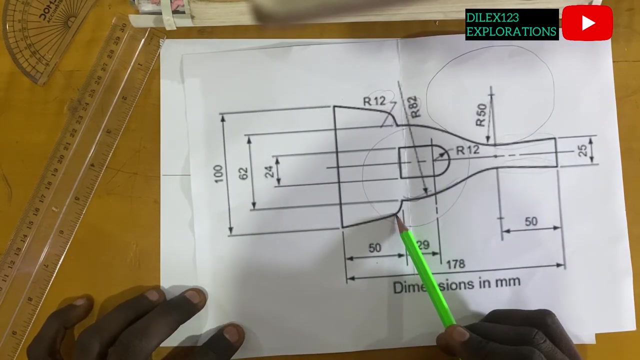 I think that is okay. now the last thing we have to do is to draw a line. so, as you can see from the diagram here, will be to join this point to this circle we drew, or the arc we drew, and we also do same for the top there. so let's.